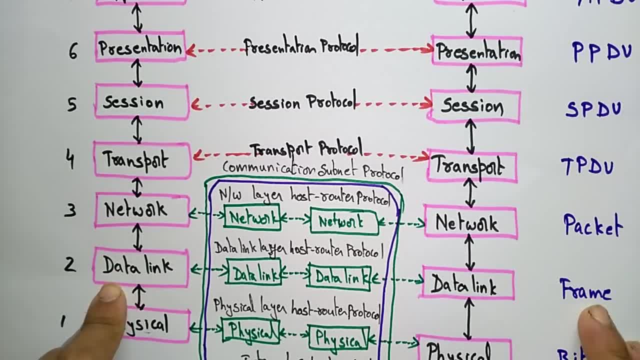 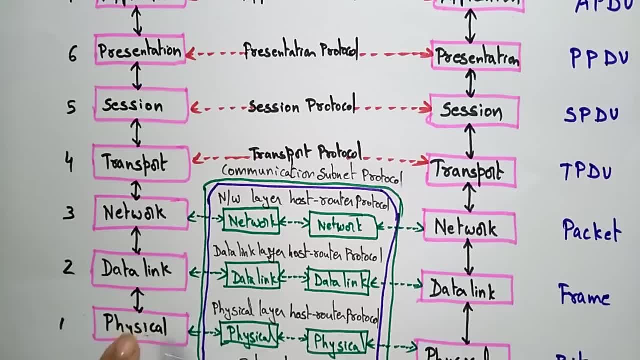 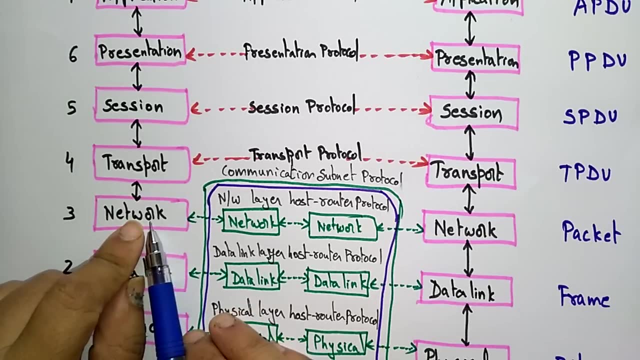 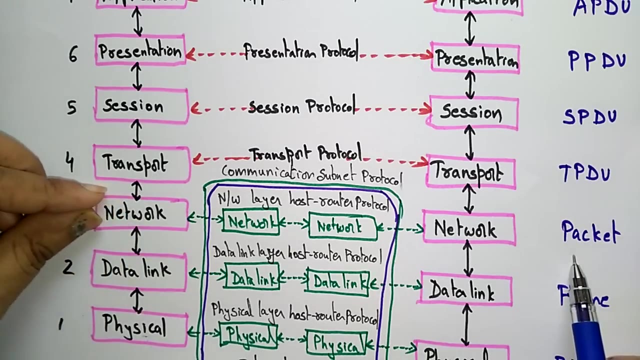 To the physical. This data link layer is having the data in the form of frames. The data will store in the form of frames, So here in the form of bits, ones and zeros, And here it is in the form of frames. And coming to the network, A network layer, This is a third layer, So here the data will be in the form of packets, So number of packets, Everything the information is stored in the form of packets. So this network data link and physical layer, 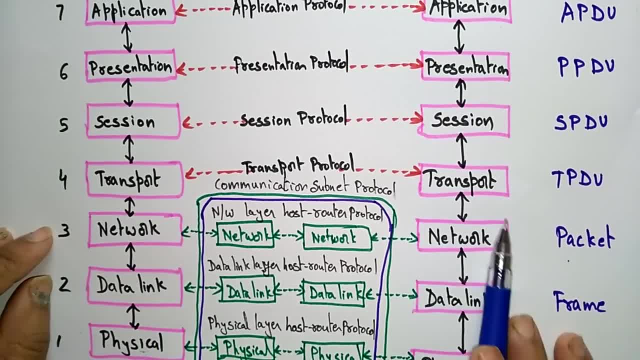 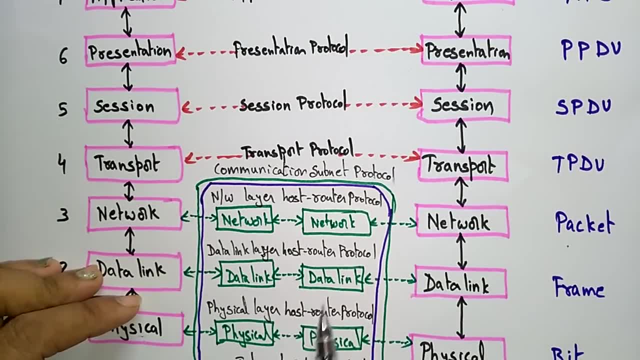 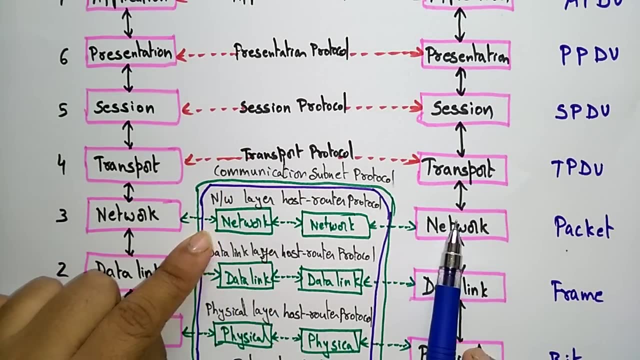 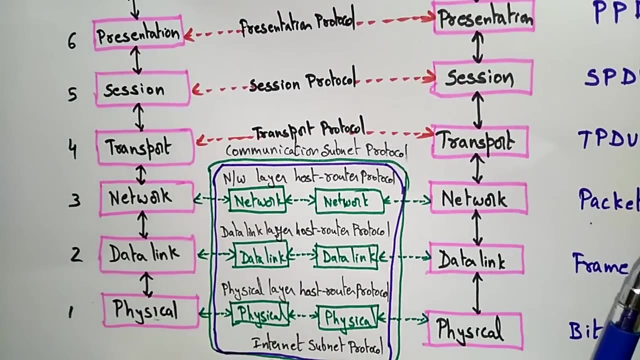 Is having is communicating with the host A to host B with the help of some communication subnet protocol. So this is a subnet router, just like a router. So it is subnet protocol. So this network layer, This is a host router protocol. data link layer, host router protocol and the physical layer, host router protocol. So this is a internet subnet protocol. internet subnet protocol and. 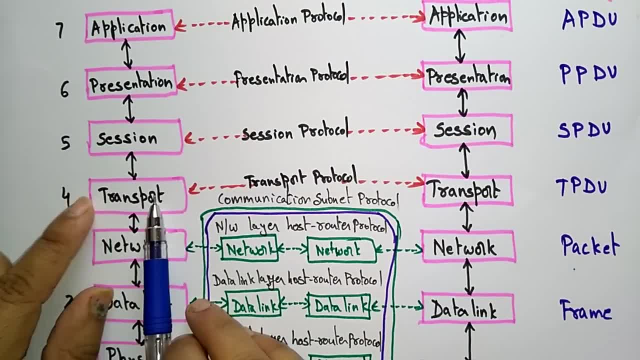 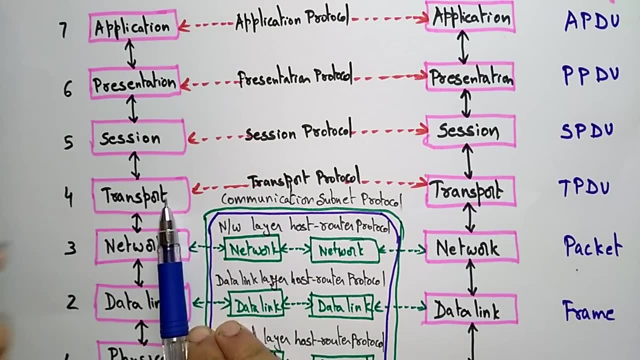 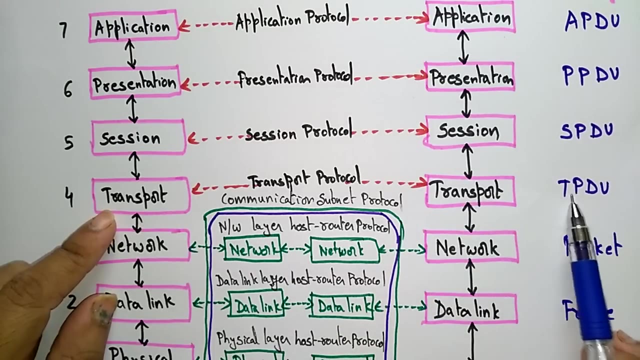 communication. Coming to the transport layer, So the transport layer is one of the important layer in the OSI reference model. So this you can call it as the heart of the OSI reference model. This is a main component which is main layer that is transporting the data. So here the name of unit exchange in the transport layer is TPDU: transport protocol data unit and session session layer is for like a 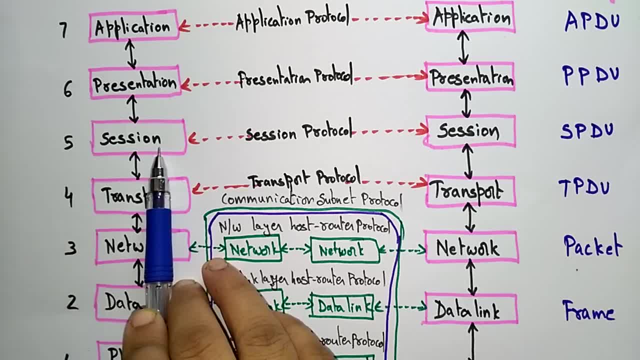 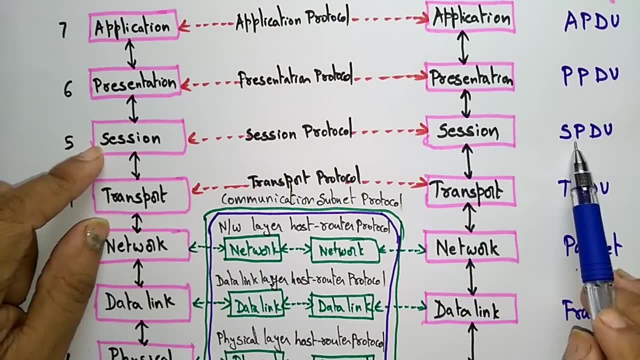 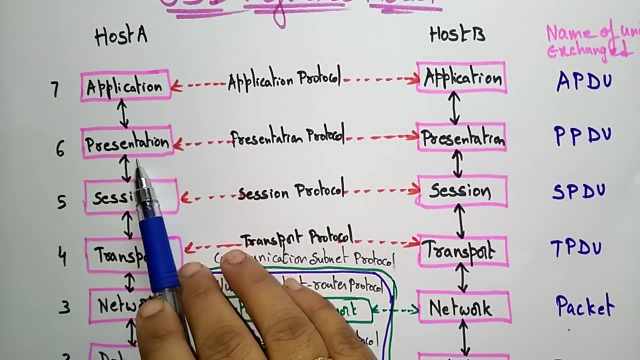 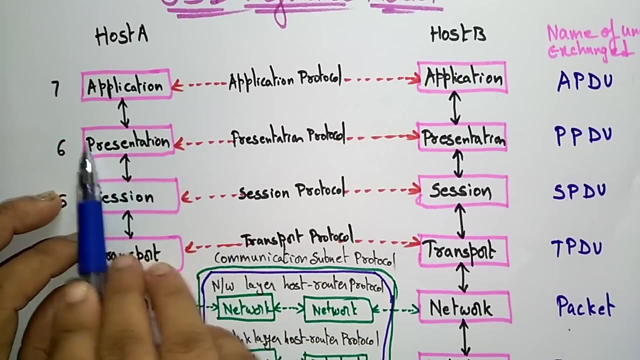 encryption. decryption means a session will be assigned to each information that is coming from the presentation layer, The session. the name of unit exchange here is session protocol data unit. Next is a presentation. The sixth layer is a presentation. The presentation layer is: is there just a translation? So whatever the application program is sending the information here, it is going to be translate to whatever the code that application layer is sending. So in the 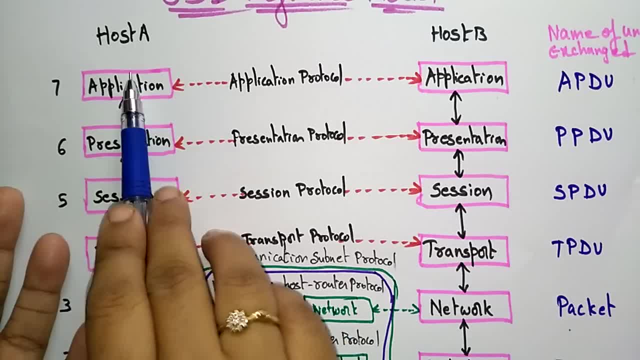 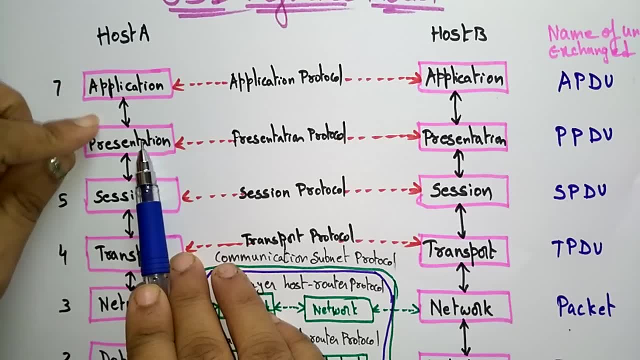 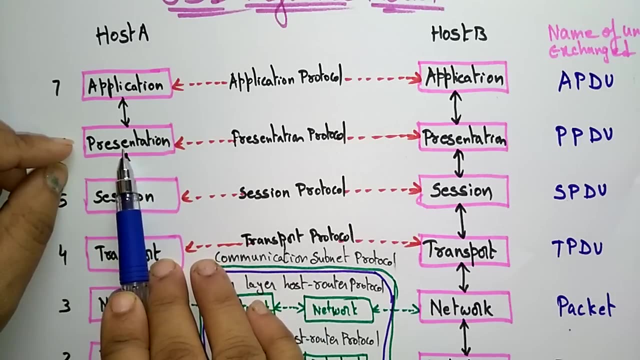 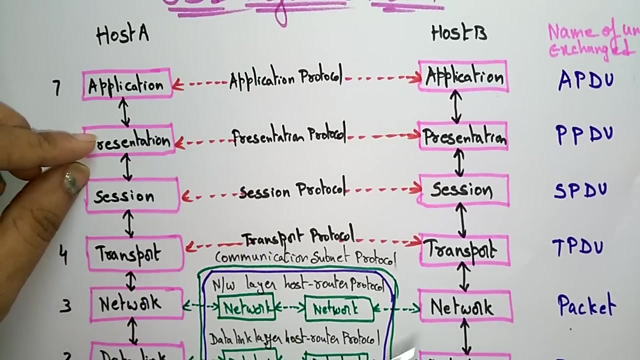 it represents in another form, another code. okay, and this code and this code will be different means the meaning is the same. but here, whatever we are sending, the application, program, application protocol, so here the presentation is, representation is different. it is all encrypted and decrypted form. then if you, if the information want to send to host b, it is in encrypted form. if it is,